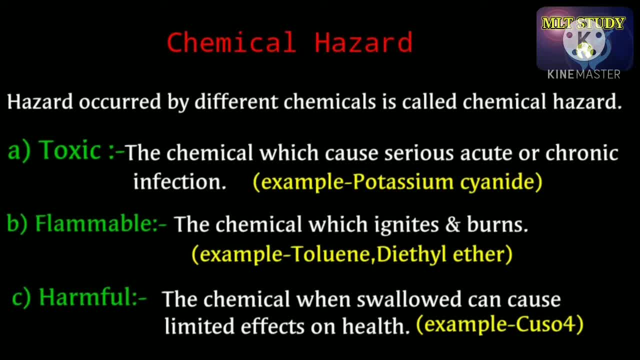 ether. Number three: harmful. A harmful substance is one that can cause limited effects on health when inhaled, swallowed or absorbed through skin. Tib carried as test tube size of 1.4in. amount, irreversible- Overall 16 Lazer conductive. 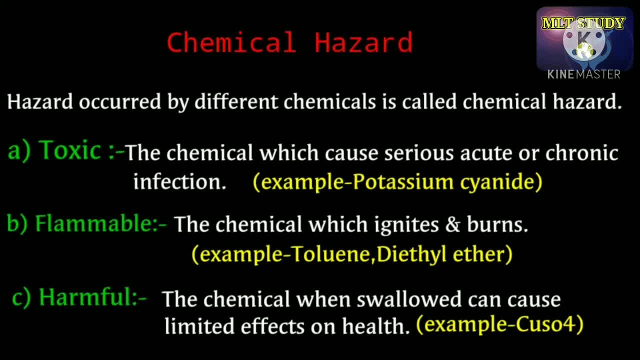 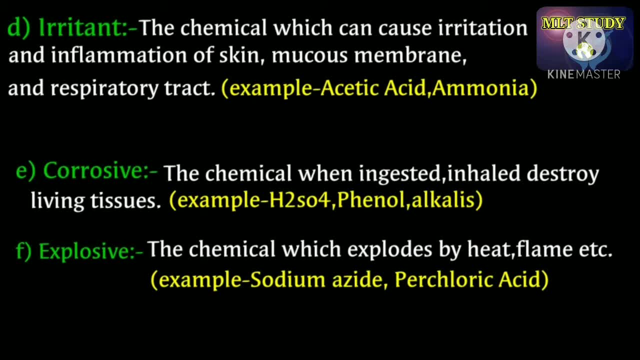 Oliver's vectors are等WORLD levels in temperature from dress temperature numbers, example: copper, sulfate. number four: irritant. an irritating chemical is one that can cause inflammation or irritation of skin, mucous membrane and respiratory tract. this includes ammonia solution, acetic acid, etc. number five: corrosive. a corrosive chemical is one that, when 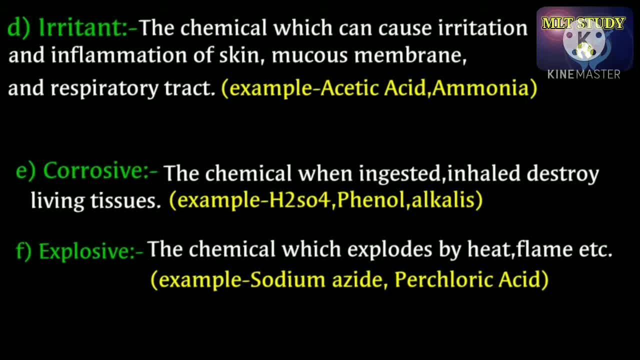 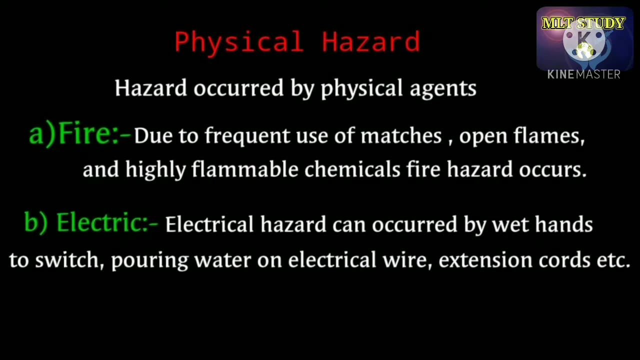 ingested, inhaled or allowed to come in contact of skin can destroy living tissues. example: so many acids and alkalis. number six: explosive: the chemical which explodes by heat, flame, etc. example: sodium, azide, perchloric acid. physical hazard: hazard occurred by physical agent. there is two types of physical hazard. number one: fire hazard. 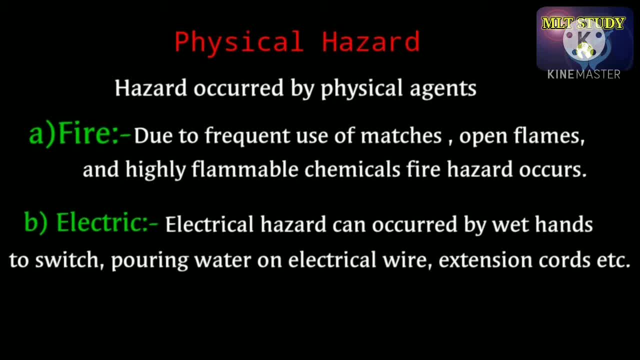 and number two electrical hazard: fire hazard. a significant fire risk exists in small laboratories due to frequent use of matches and open flames, and highly flammable compound is also responsible for the fire risk in the laboratory. number two: electrical hazard. electrical hazard can occur by touch the switch on weight hands. 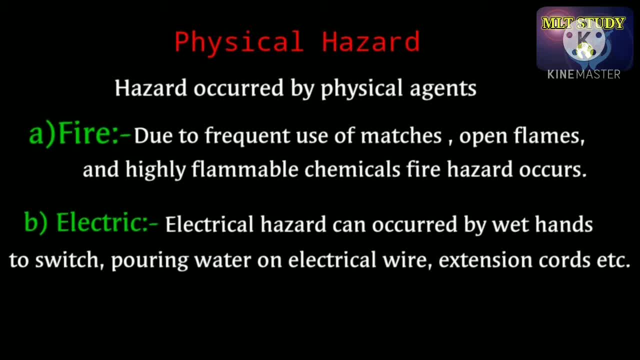 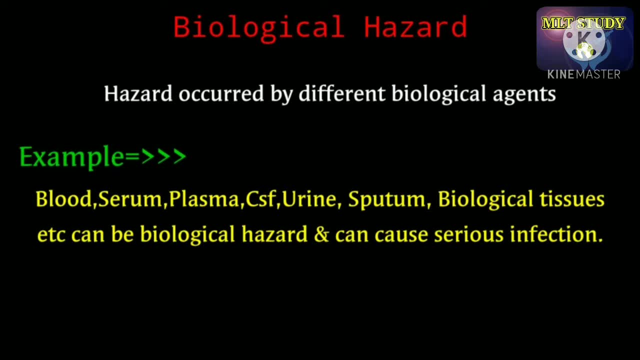 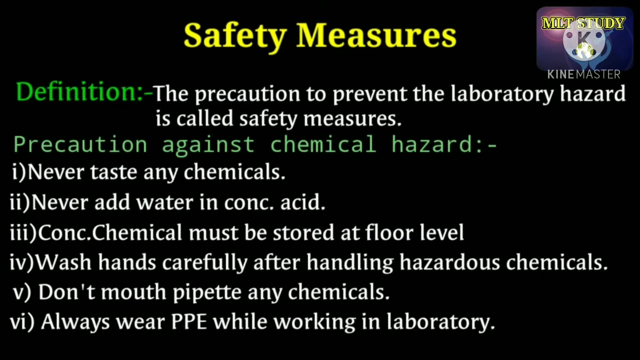 pouring water on electrical wear and fried extension cord. it is a biological hazard, hazard occurred by different biological agent like whole blood, plasma, serum, cerebrospinal fluid, urine, sputum, etc. and these can cause infection of hiv and hepatitis viruses. next septum: 7 safety measures in vascotticCOM. 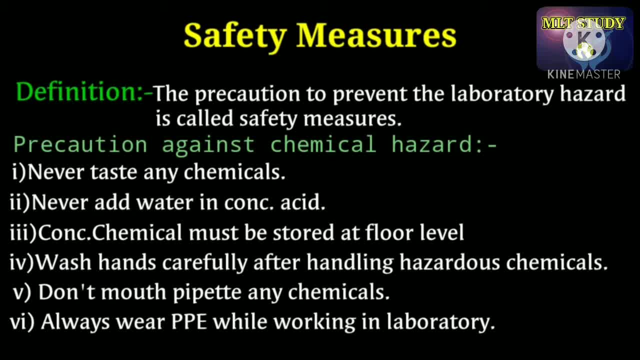 1. safety measures are listed in second. safety measures are listed in safety measures. safety measures are the precaution to prevent the laboratory hazard. first the precaution against chemical hazard. never drove any chemical. never add water in concentrated acid. chemical must be stored at floor level. wash hands carefully after handling. 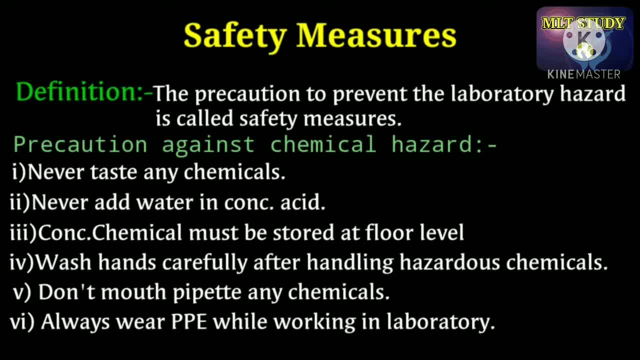 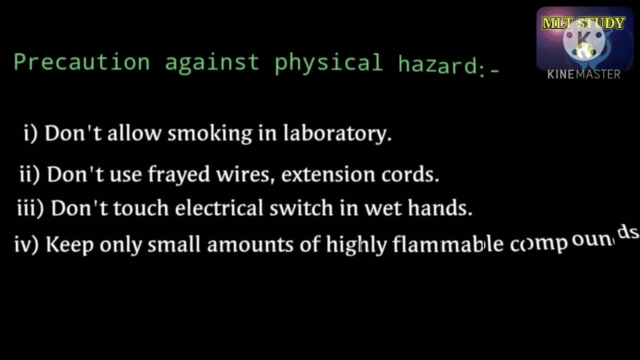 hazardous chemicals. do not mouth pipette any chemicals. always wear personal protective equipment- PPE- while working in laboratory. this PPE includes gloves, face mask, laboratory apron, covered shoes, eye goggles, ETC. second precaution against physical hazard: do not allow smoking in laboratory. this will prevent the fire hazard. do not use pride wears extension cords. do not touch electrical. 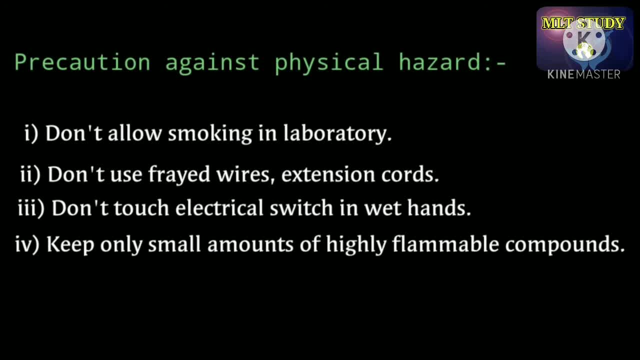 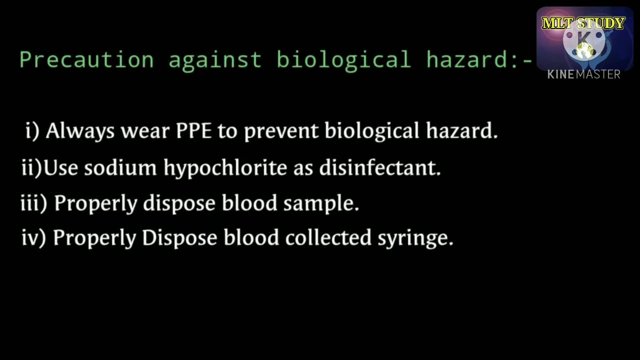 switch in the weight hands. the second and the third point will prevent the electrical hazard in the laboratory. keep only small amounts of highly flammable compounds. this will prevent the fire hazard in the laboratory. and third, precaution against biological hazard. always wear PPE to prevent biological hazard. 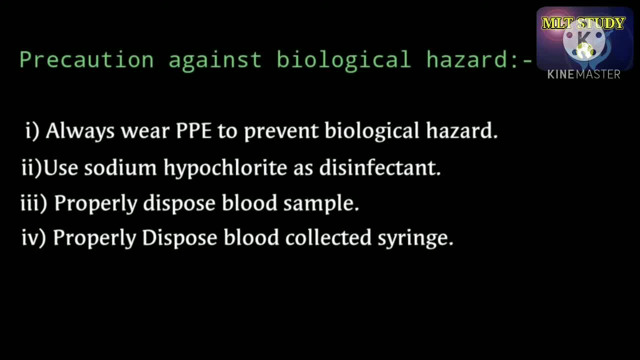 and use sodium hypochlorite solution as disinfectant, properly dispose blood sample and blood collected syringe. so these are the safety measures that are taken against the laboratory hazard, physical hazard, chemical hazard and biological hazard. if the video is useful, please subscribe to my channel and hit the bell icon and you will get all news of upcoming videos. Thanks for watching. 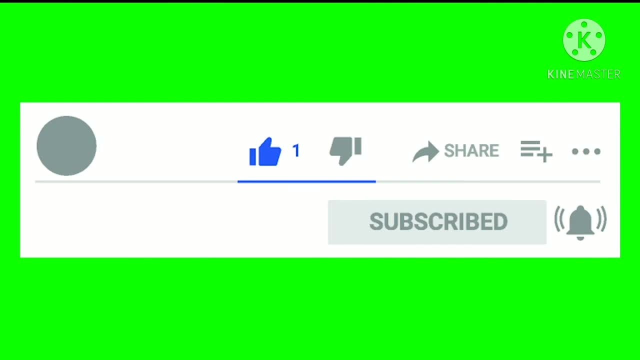 helpful to you. please subscribe my channel and press the bell icon to get the notification.